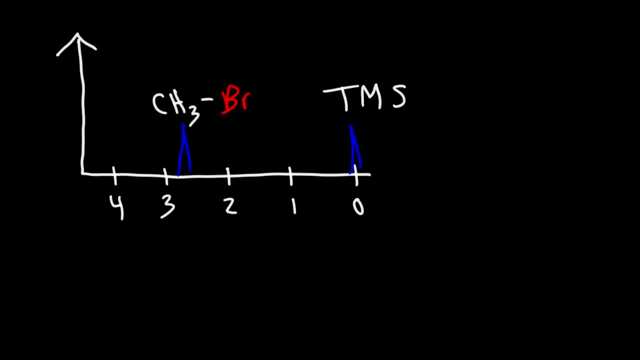 In this video we're going to talk about chemical shift. Chemical shift, represented by the symbol delta, is basically the ratio of the observed chemical shift, which is typically given in hertz, divided by the operating frequency of the spectrophotometer, which is typically 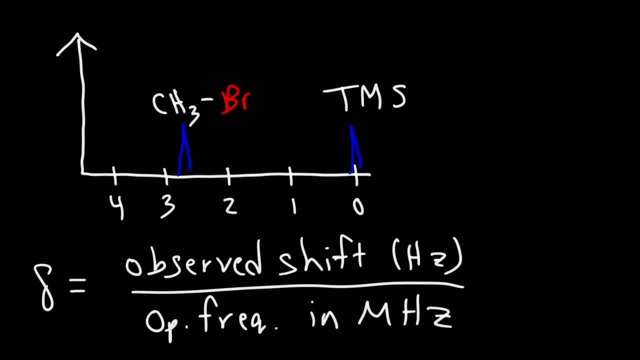 given in megahertz. Now, to get a number between 0 and 12, you're going to have to multiply this by 10 to the 6th. Now, on the x-axis, these represent chemical shift values for different signals and the unit is ppm- parts per million. Now what we have here is a reference. 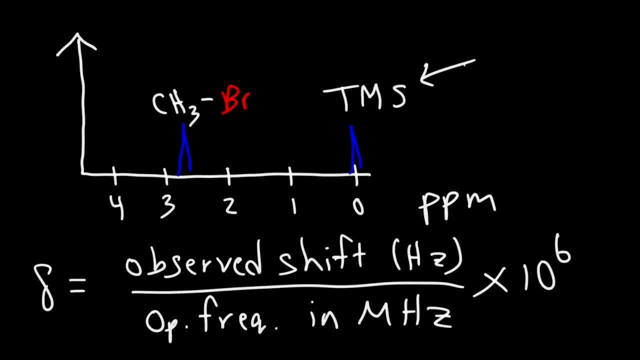 signal. TMS, also known as tetramethylsilane. It's basically a silicon atom with four methyl groups. On the right we have methyl bromide. Now notice that methyl bromide has a higher chemical shift than TMS. The reason for that is because bromine is more electronegative than silicon. 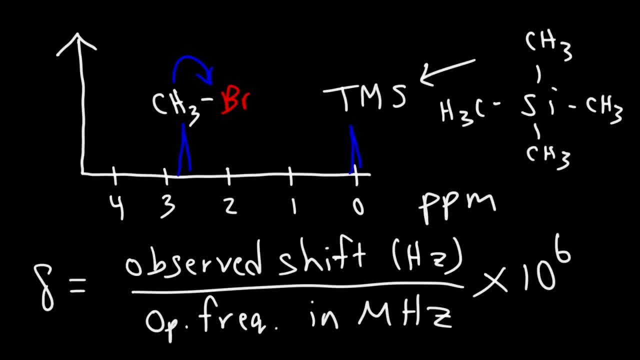 Because the protons are next to an electron withdrawn group, they will have a higher chemical shift. Thus they will appear downfield on the NMR spectrum, which is basically the left side. Upfield is towards the right side, The protons that are shielded to an external magnetic. 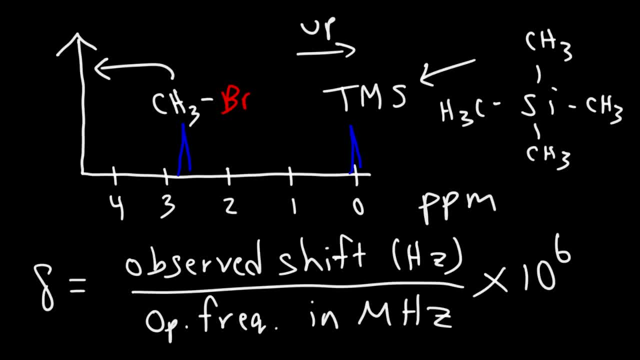 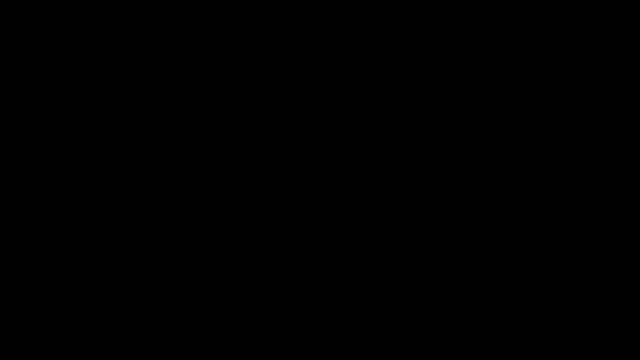 field, they will appear upfield. The ones that are deshielded will appear downfield, which is due to the presence of an electron withdrawing group. So here's a question for you. Let's compare methyl bromide with methyl chloride. 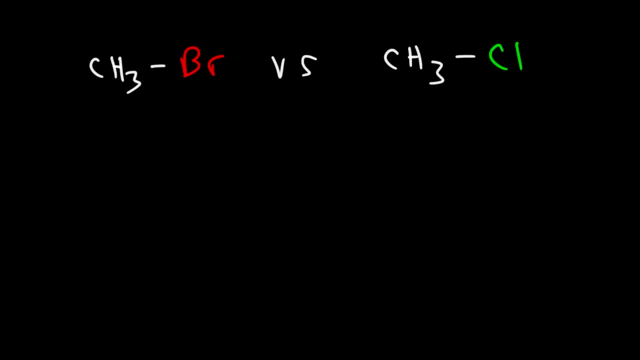 So, dealing with HNMR, which one will have a higher chemical shift? Would you say it's the protons in methyl bromide or the protons in methyl chloride? Because bromine is more electronegative than chlorine, methyl bromide should have a higher. 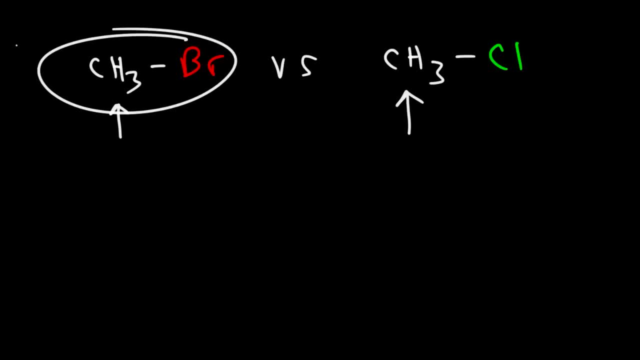 chemical shift than methyl chloride. So when dealing with the halogens, here's what you need to know: Andessen Running 보 acabar в ig Corеров iskt chemical shift. and then it's going to be methyl chloride, followed by methyl bromide, followed by methyl iodide. so 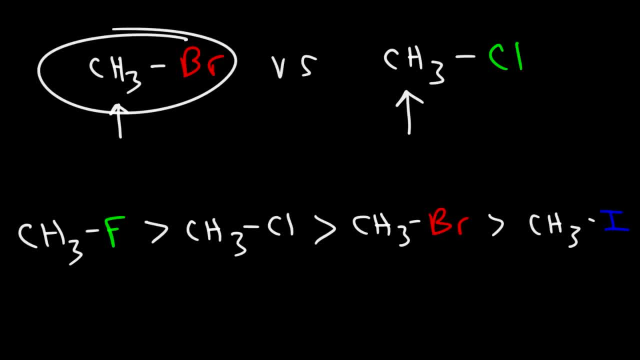 this is due to the inductive effect. so the proton that's attached to a carbon with a more electron negative atom attached to it, it's going to have the higher chemical shift. it's going to appear more downfield now, according to one textbook. here are the values for: 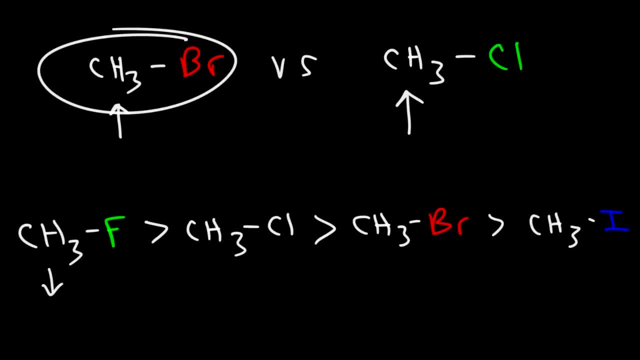 these compounds. so the chemical shift: for methyl fluoride, that is, the protons on it, it's about 4.3 ppm, or parts per million. for methyl chloride it's 3.1. for methyl bromide it's about 2.7 and for methyl iodide 2.2. now for methane, if you. 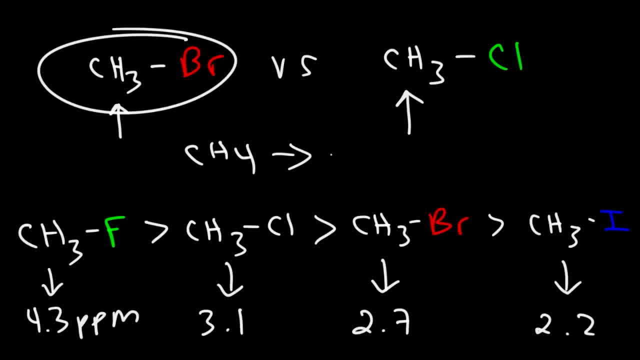 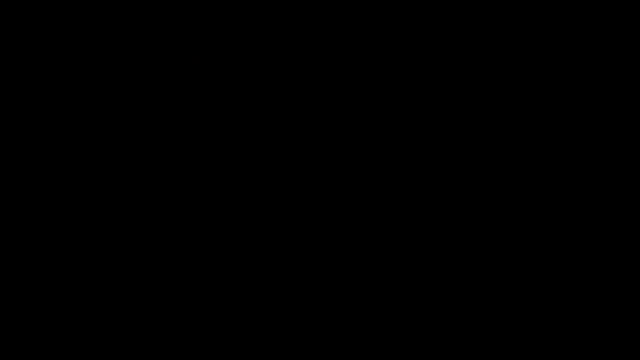 want to compare that to methyl iodide. it's much less. it's going to be about 1.0 ppm. so the presence of a halogen will greatly increase the chemical shift of these compounds. now the next thing that we need to mention, which is obvious: 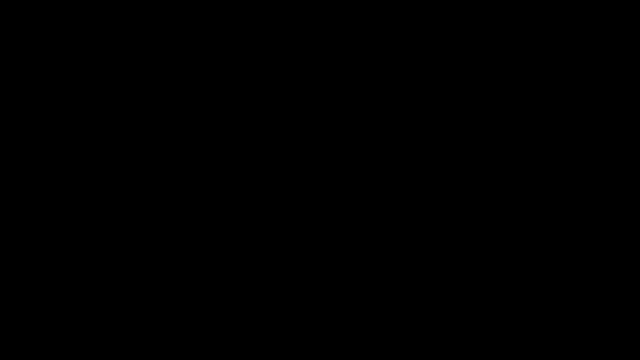 in nature, but it's good to see it- is that if the number of electron groups- i mean, excuse me, electron withdrawing groups- increases, the chemical shift will increase as well. so in this example we have three chlorine atoms and the chemical shift for this proton is 7.3 ppm. now we're 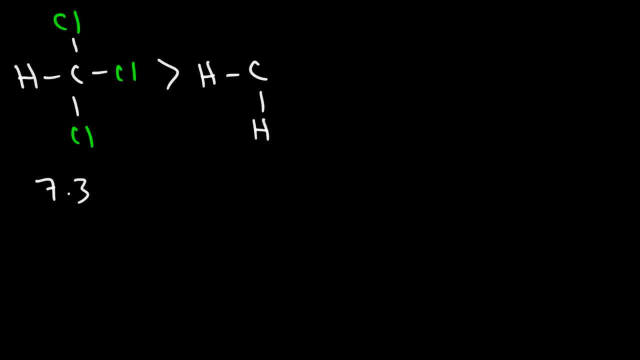 going to compare it if we had two protons on this carbon instead of three. so the chemical shift for dichloromethane is about 5.3 ppm. and then let's compare that to methyl chloride, which we said was 3.1, and methane, which is about 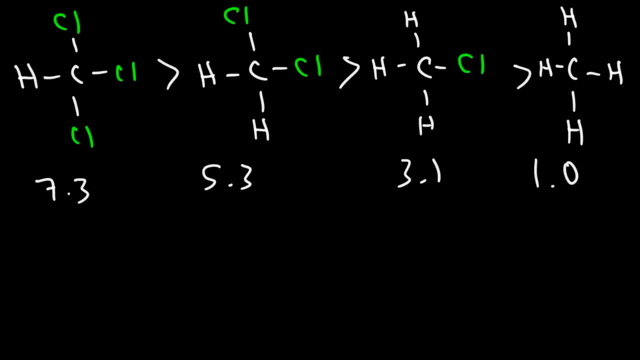 1 ppm. so, as you can see, the more halogens or the more electron withdrawn groups that you have on a carbon atom, it's going to basically pull the electrons from the carbon atom. that's making this proton deshielded towards an external magnetic field. that's increasing the chemical. 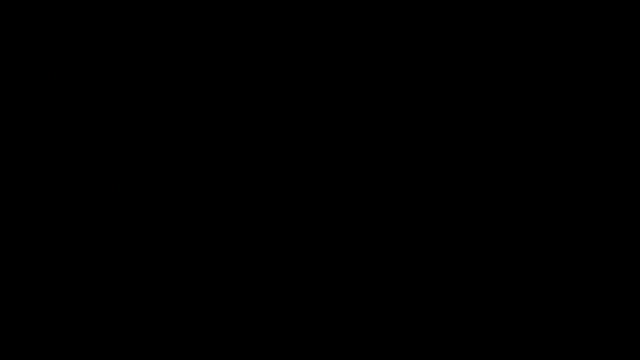 shift of that proton on an NMR spectrum. now the next thing we need to talk about is the position of the protons relative to an electron withdrawn group in a molecule. so here we have nitro propane, or you can say one nitro propane, and there's three different types of protons. 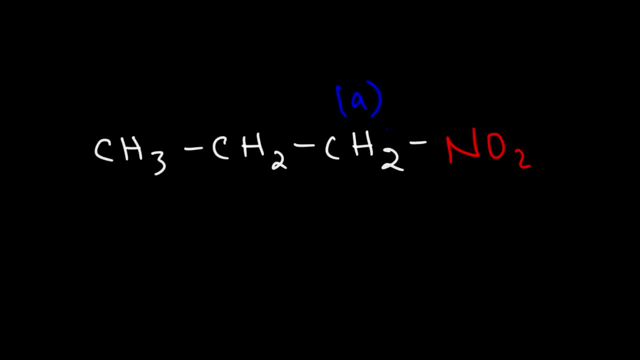 the two protons in this CH2 group will generate one type of signal and then these two protons will generate another and then these three will generate a different signal. so in the NMR spectrum will have three different signals for this molecule. which proton will have the? 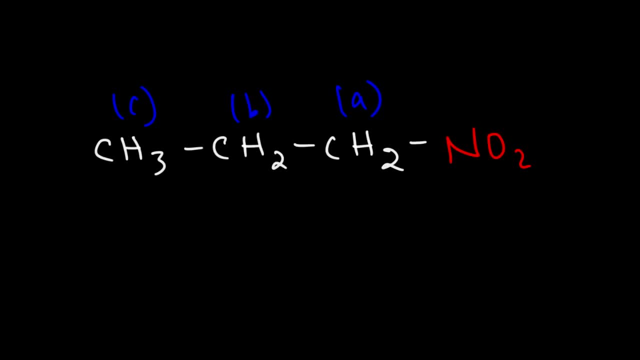 highest chemical shift and which one will appear the most downfield in an NMR spectrum? would you say it's the protons corresponding to signal a, signal B, or the ones corresponding to signal C? what would you say now? keep in mind the NL2 group, the nitro group is a powerful 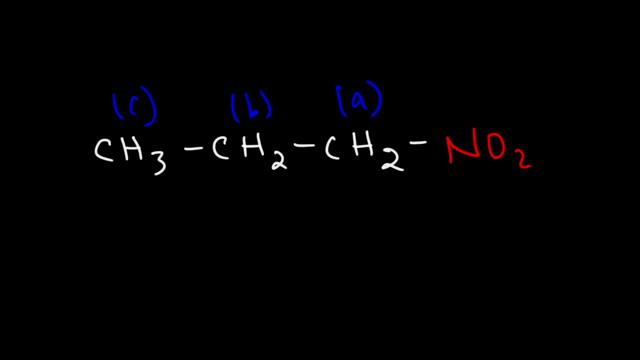 electron withdrawn group. now the answer is, of course, the protons nearest the electron withdrawn group. so signal a is going to have the highest chemical shift. signal C, because it's furthest away from the nitro group, it's going to have the lowest chemical shift. so the number 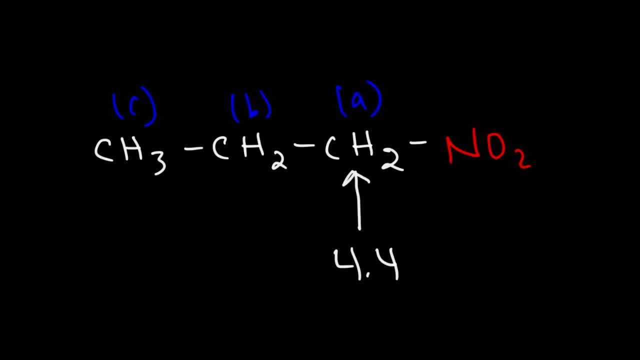 correspondent to this is going to be about 4.4 ppm and for the methylene group in the middle it's about 2.1 and for the methyl group at the end, 1.0. so the nitro group is still able to affect the. 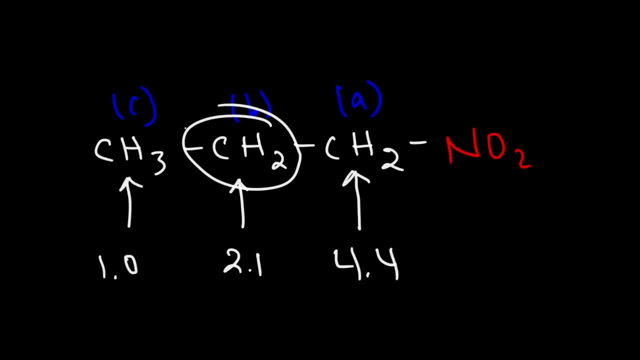 protons correspondent to signal B, even though it's not directly attached to that cardin now the methyl group. that is very far away from this electron withdrawn group. it's not really affected as much. so as you can see the relative position of the protons next to electronic withdrawn. 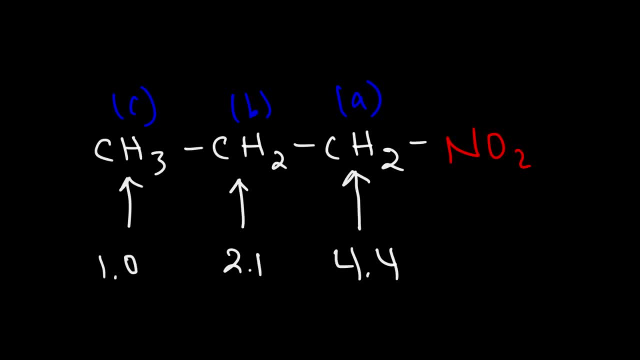 group has an effective one, the static. those that are closest to the electron walk drawn group and have the highest chemical shift, the ones that are furthest away. they will have the lowest chemical shift because we're talking about the. they will appear upfield, while these will appear downfield. now let's work on. 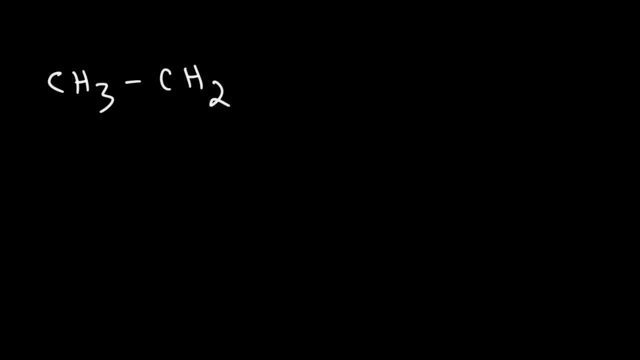 another example. this one is going to be a little more challenging than the previous examples. so here we have a molecule of butanone. which protons will be the most deshielded? the ones corresponded to signal a, signal B or signal C? what would you say? feel free to pause the video and work on this now. the electron withdrawn group is undoubtedly the carbonyl group, and because protons C is farthest away from it, this is not going to have the highest chemical shift. in fact it's going to have the highest chemical shift in the electron group. so the battle is between signal B and signal A, both of which are equally. 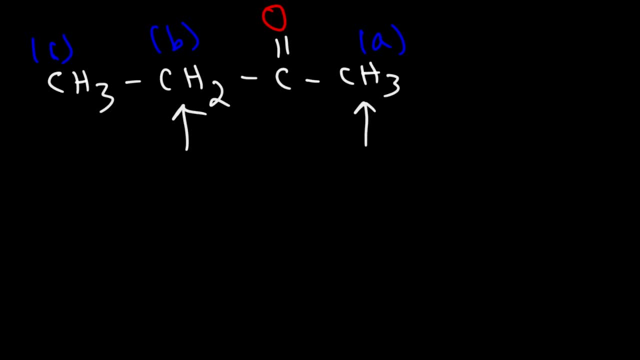 distant from the carbonyl group. so now, which one is going to be the answer? before we can understand which signal is going to have the highest chemical shift, we need to talk about something. what you need to know is that, let's say, if we have a carbon, 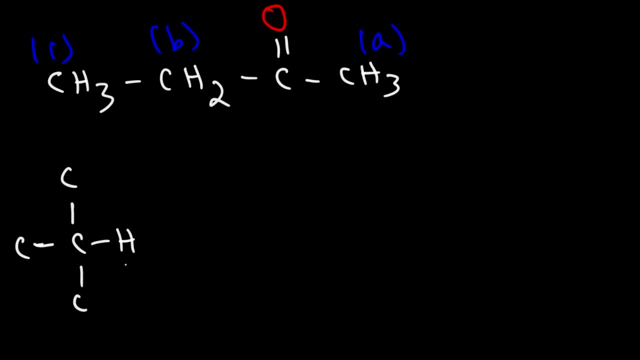 with one hydrogen atom. so this is called a methane proton, which is attached to basically a tertiary carbon. the methane proton is going to have a higher chemical shift than a methylene proton, which is basically a CH2 group. so I'm going to write it here: methylene. the methylene protons are attached to a secondary carbon because that carbon is attached to two other carbons and those protons will have a higher chemical shift than a methyl proton, which is basically a CH3 group. in this example, the methyl protons are attached to a primary carbon and just to give you some numbers: methyl- protons, the signals are usually around 0.9 to 1.1. now these can vary based on the molecule, but that's like a rough estimate. the methylene protons are usually about 1.2 to 1.3. the methane protons could be anywhere from 1.4 to 1.7, but we need to. understand is that the protons attached to a tertiary carbon are more down shielded. I mean down shielded more downfield then the secondary once, and that's more downfield then the protons that are attached to a primary carbon. now the question is why? why are the protons more? 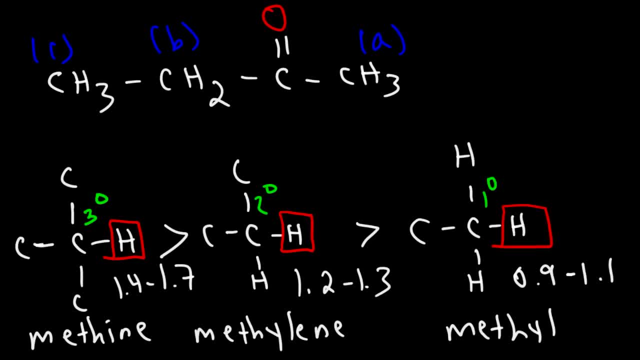 down shielded when they're attached to a tertiary carbon compared to the ones that are attached to a primary carbon, and the answer has to do with the number of electron withdrawn groups. carbon is more electronegative than hydrogen. the en value for hydrogen is 2.1 and the electronegativity value 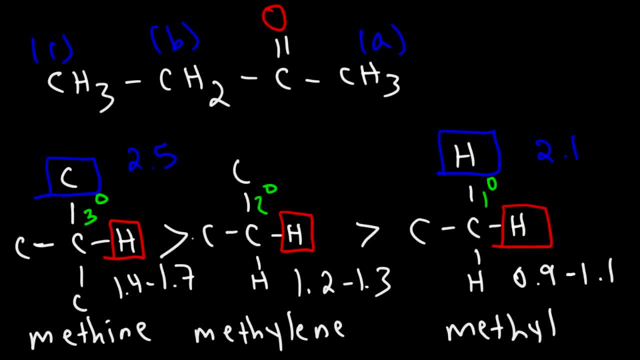 for carbon is 2.5. so if you replace one hydrogen with a carbon atom, this carbon now has more electron withdrawn groups that are pulling electrons away from it, making this proton more deshielded to a magnetic field. and so because carbon is more electronegative than hydrogen, having three carbon atoms on this, central carbon is going to have a greater deshielding effect as opposed to having just one carbon atom, and so that's why methane protons are more deshielded than the methylene protons or methyl protons. so now let's compare these two protons, the methyl protons and the methylene. 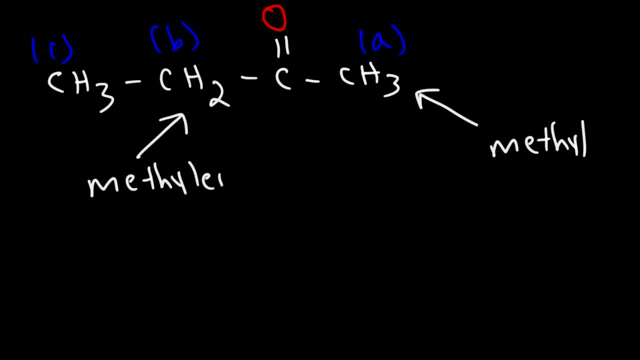 protons, based on what you know, which one is going to have the higher chemical shift. now let's compare the carbon atoms. this is a methyl carbon atom which is attached to another carbon atom, so it's a primary carbon. this carbon atom is secondary. it's attached to two of the carbon atoms and, as we know, the protons. that are on the secondary carbon. it's going to be, it's going to have a higher chemical shift than the ones in the primary carbon. so the methylene protons it's going to be more deshielded than the methyl protons. so signal B should have the highest chemical shift. then it should be. 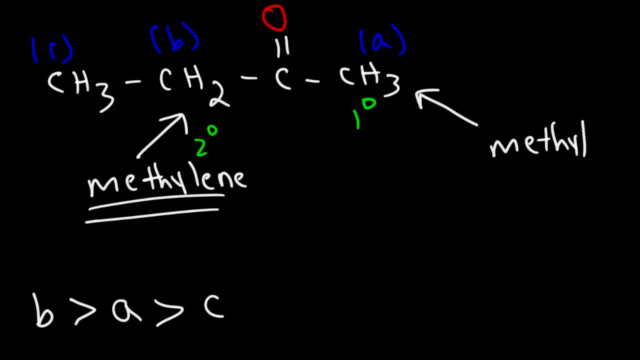 signal A and C should have the lowest. now just to put some numbers to this: the methyl proton has a chemical shift of about 2.14 parts per million. the methylene protons has a chemical shift of 2.45, a little bit more than the methyl. protons and the methyl protons at the left corresponded to signal C. they have the lowest chemical shift, which is around 1.06, and so, as you can see, the methylene protons has the highest chemical shift because there's more carbon atoms attached to this carbon. now you need to know the chemical shifts of 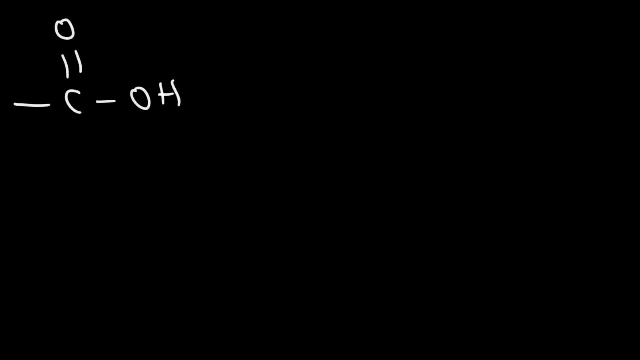 a few common functional groups. I'm not going to go over all of them but because you can look it up in a textbook, but just a few. for our carboxylic acid, the proton will have a chemical shift of somewhere between 10 to 12 parts per million. next up is the aldehyde. the aldehyde proton will have a 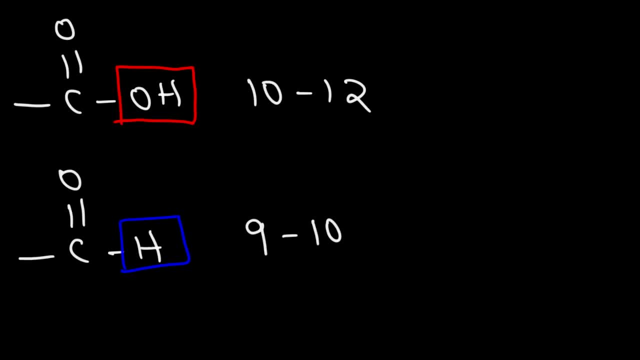 signal somewhere, usually between 9 and 10. the next one you need to know is benzene, the protons on a benzene ring. they can vary, usually between 6.5 and 8.5. now if you have a methyl group attached to a benzene ring, it's not going to have a. regular signal of a methyl group, which is usually around 1 ppm, but this is going to be more deshielded and it's going to be around 2.1 to 2.3 ppm. now, if you have a halogen represented by the letter X on the carbon with a,